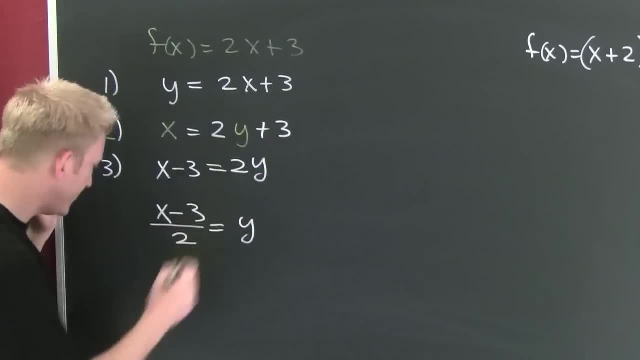 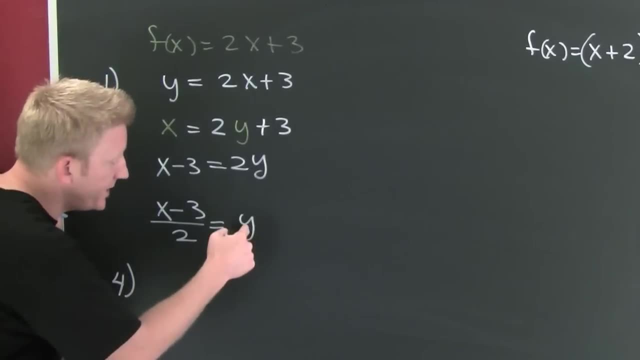 over two is equal to y. And finally, the fourth step, where I'm going to get you, I'm going to tell you- I'm taking points right here, because this is the most commonly forgotten step- You need to interchange y with f inverse. 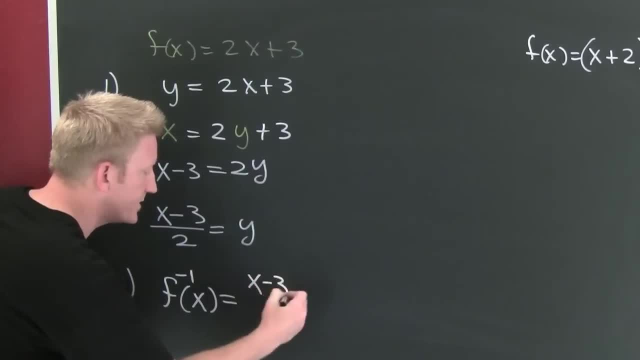 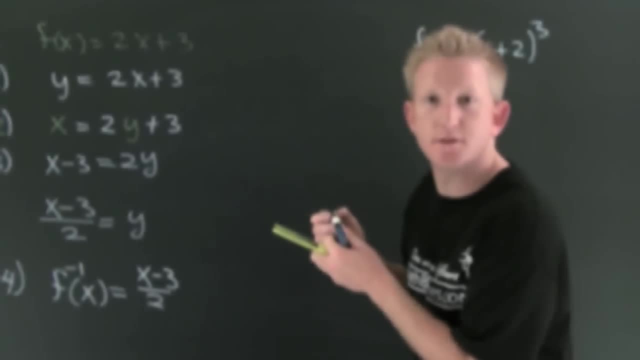 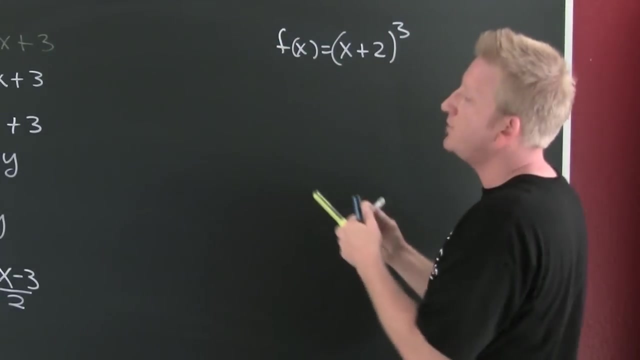 f of x, And then that's equal to an x minus three over two. Oh, Moving on to my next one, Yes, My contacts blurry, I don't know. I'm back up here, Okay, Following my same processes, Uh-huh, Okay. 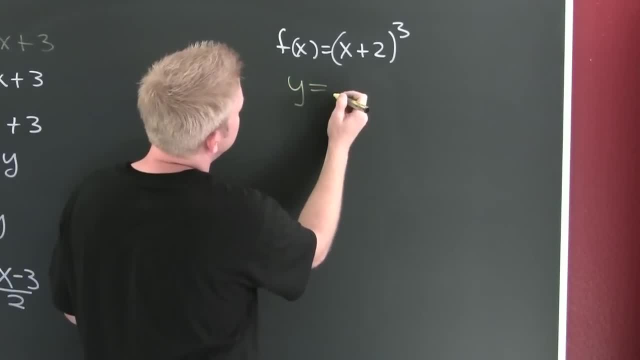 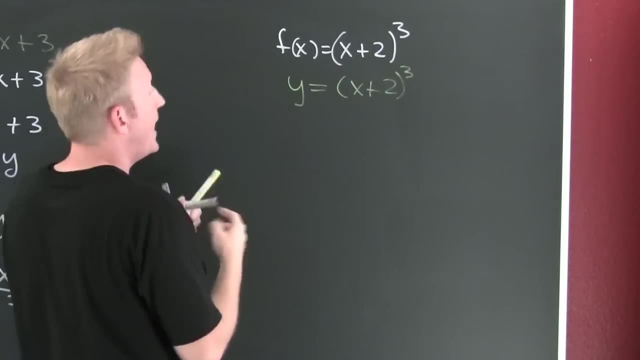 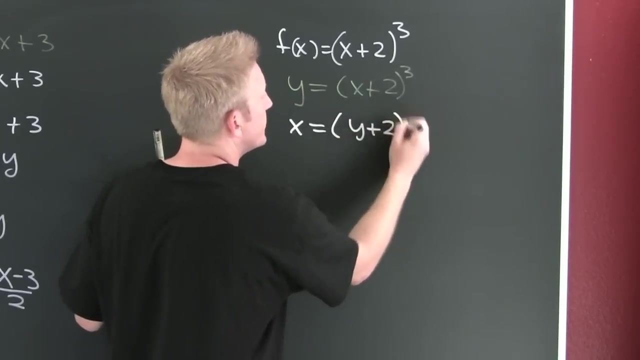 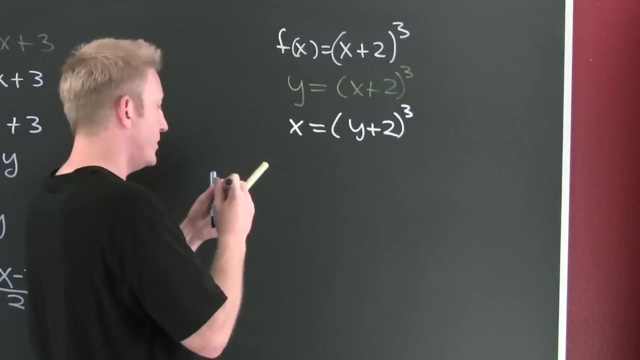 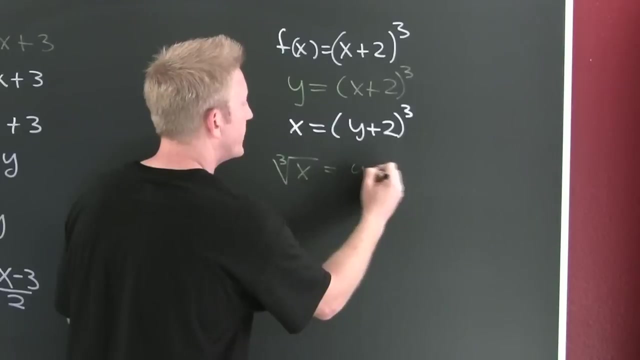 Okay, Interchange f of x with y, Yes, And then this is x plus 2y. Oh, Oh To the third power. Now I want to interchange x and y. I'm going to let x equal y plus two. Oh To the third. Now you need to solve for y. That means you need to take the third root of both sides. What you do on the one side, you must also do on the other. Here I have the third root of x is equal to y plus two. Come on, marker. 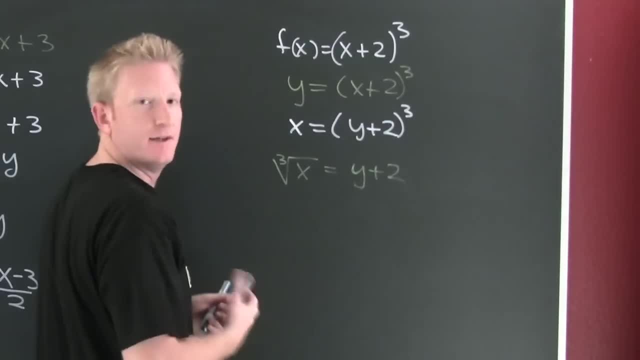 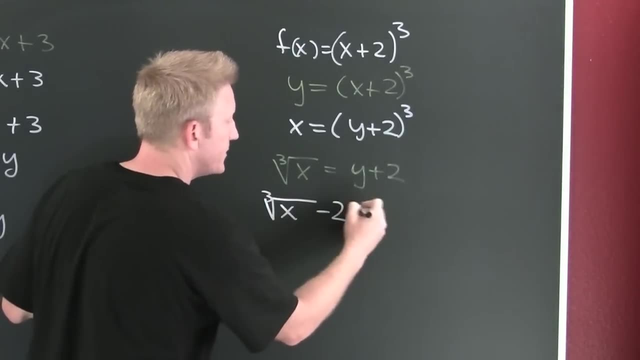 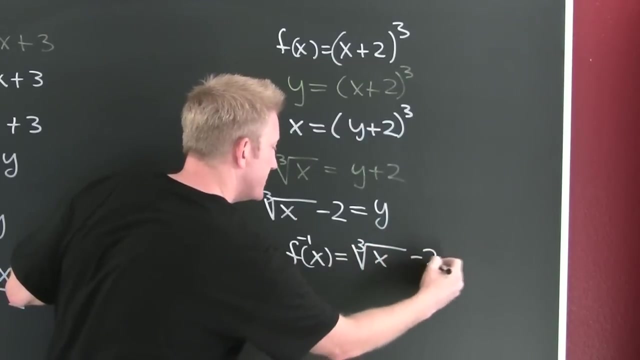 Wow, I hate it when they just quit on you like that. Okay, Yes, Subtract off that two. This is the third root of x minus two is equal to y. Very nice, Um, So then last step: F, inverse of x, is equal to the third root of x minus two. And then: 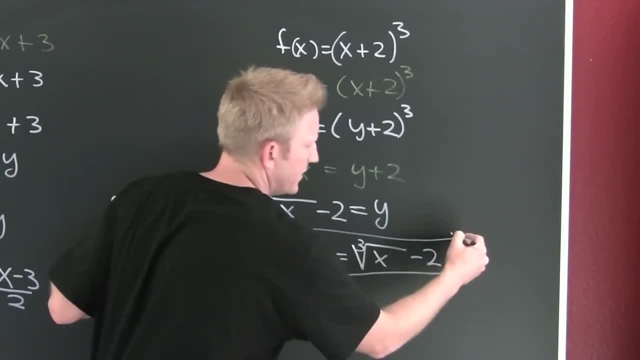 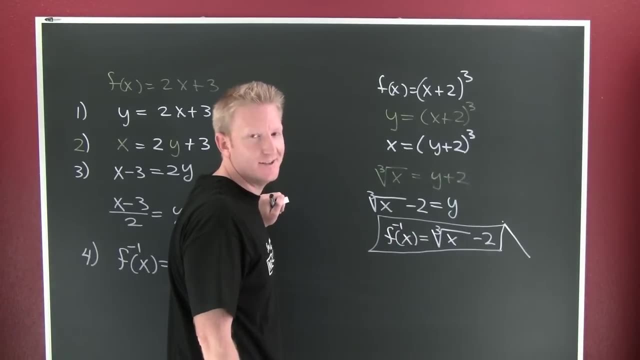 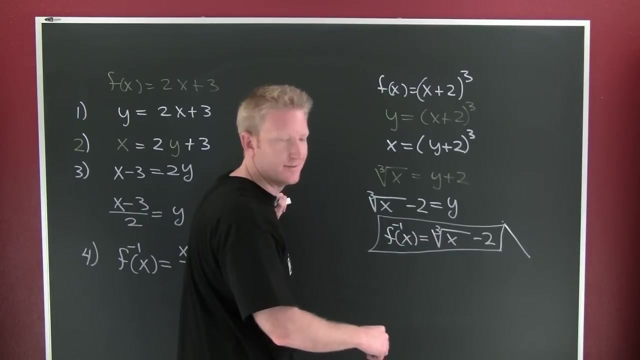 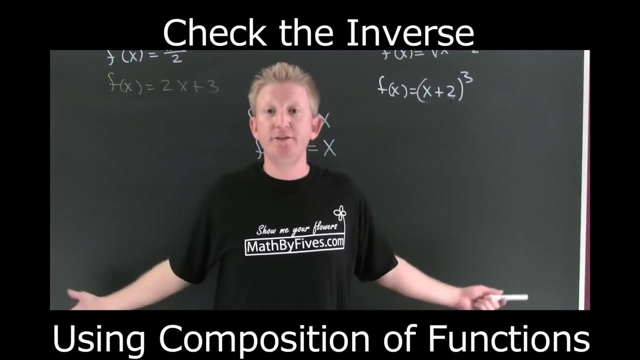 A box. Oh, That's not a flower. What is that? It's a tent. Do you know why? Because that last problem was in tents And a flower. But if you don't believe me, check it. How do you check whether or not you found inverse was the actual inverse? Well, there's a property of inverses. I don't know. 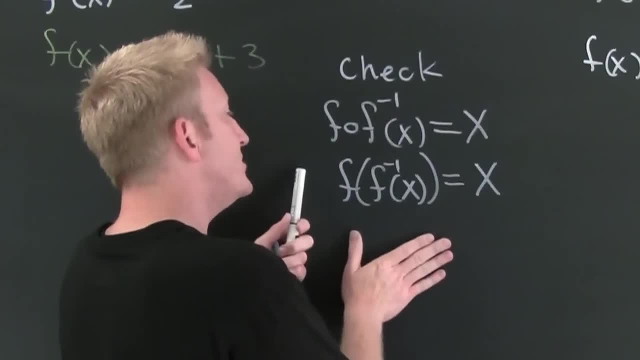 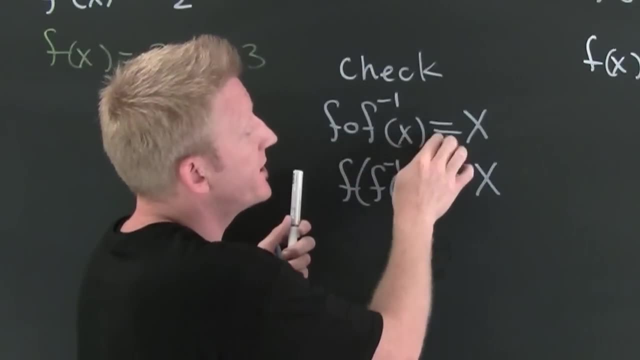 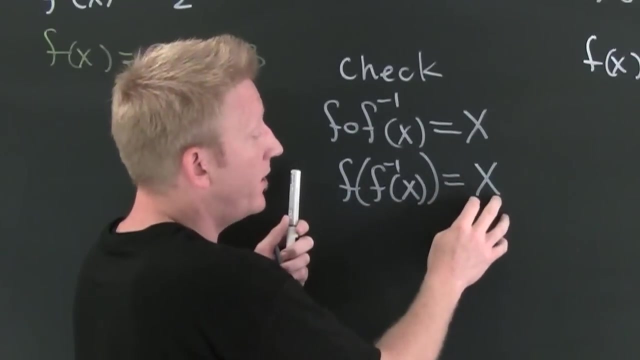 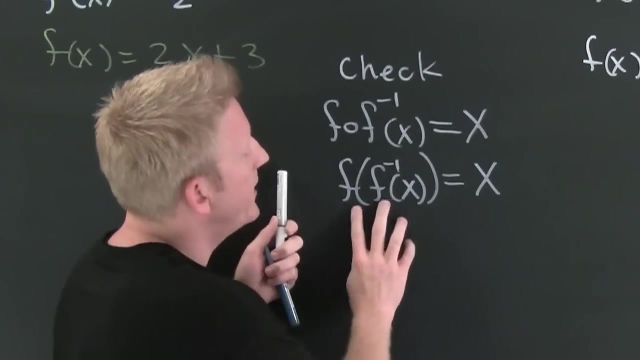 Uh huh, Okay, And this is the property To check it. you're going to check the composition of the two, The inverse and the function. Yeah, F of f inverse is going to spit out the argument. If it's the inverse, F of f inverse is the argument. Composition: If you want to check out composition, look at the composition video. Yes, Um, It also goes both ways Right Here in these algebras: Um, Our left products and our right products. 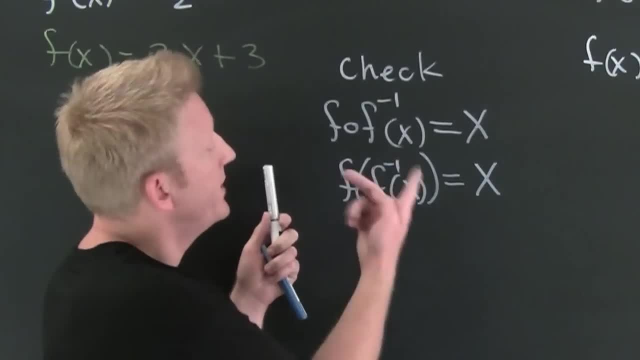 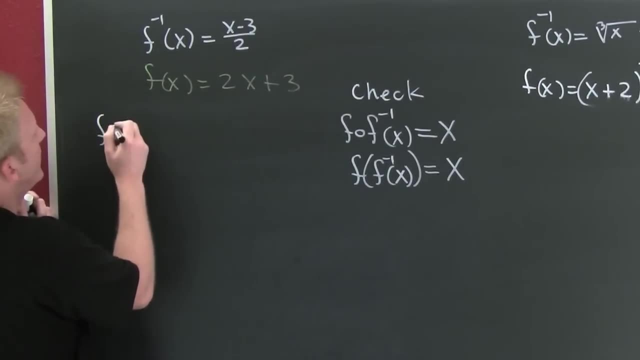 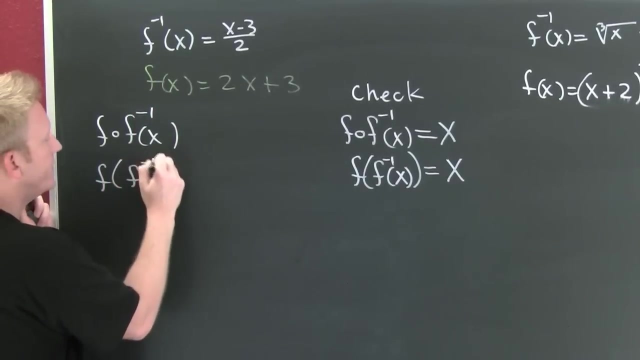 And our right products are the same, But that's not true with all algebras. So then you'd want to, you know, check it both ways. Okay, Yes, Up here To this example. Let's look at f of f inverse of x. This is going to be f of f inverse of x. This is going to be f of My f inverse was found to be x minus three divided by two. Oh Yes, So then, 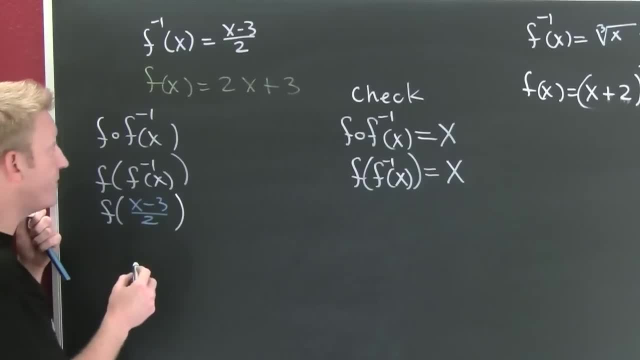 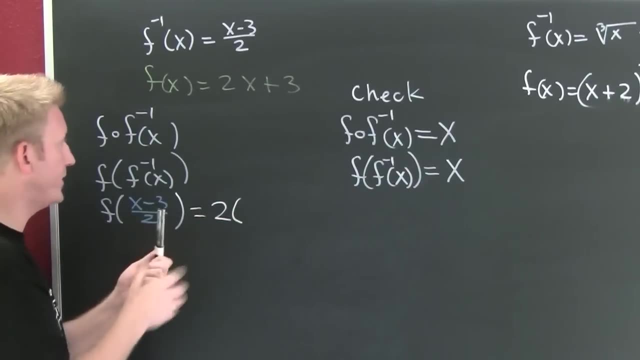 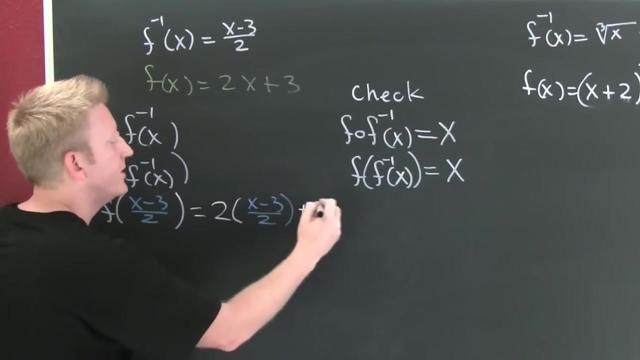 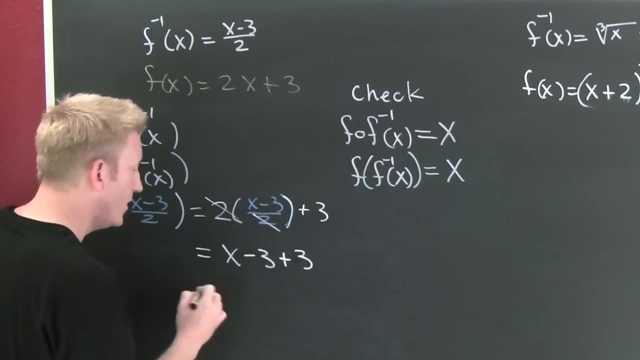 Everywhere I see an x, An f of x. I'm going to put this So sure, This is going to be two times, Wait for it. X minus three, divided by two. Yes, In addition to that, I'm going to put a three, Okay, Divide. And then I have x minus three plus three, Oh, And we see, We do get our arguments. So then we can conclude: Yes. 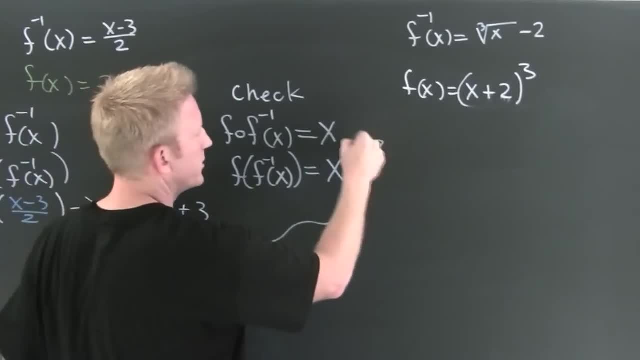 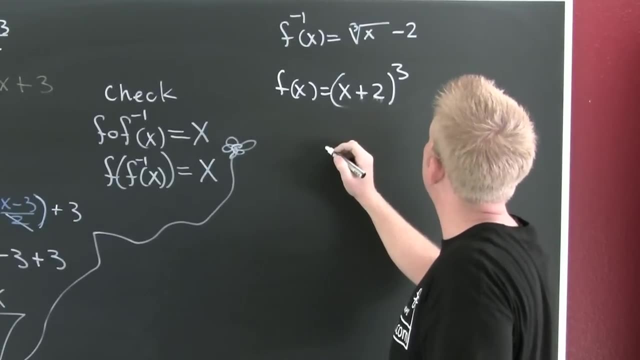 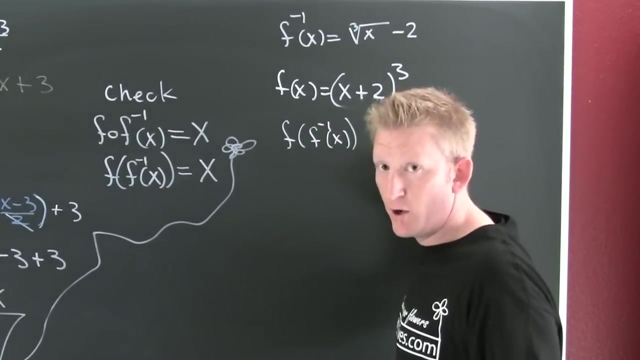 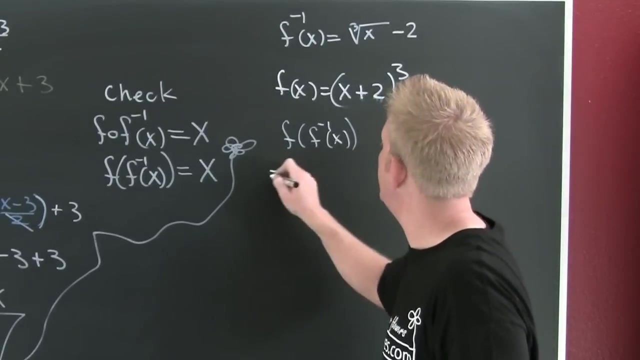 Inverse. Bringing me on up here, I'm going to check that composition once more Once again. Oh Yes, I'm looking at f of f inverse of x. If I compose the two And it does give me the arguments, or x the identity himself, Then we do have inverses. So then I'm looking at f of. I found That's an awful flower, I found. 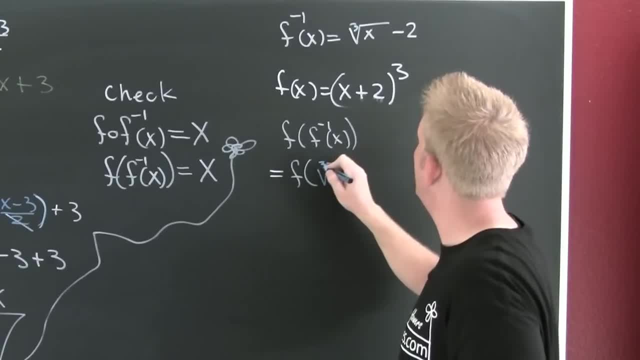 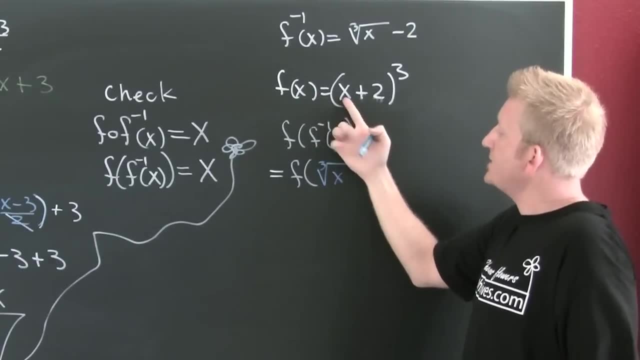 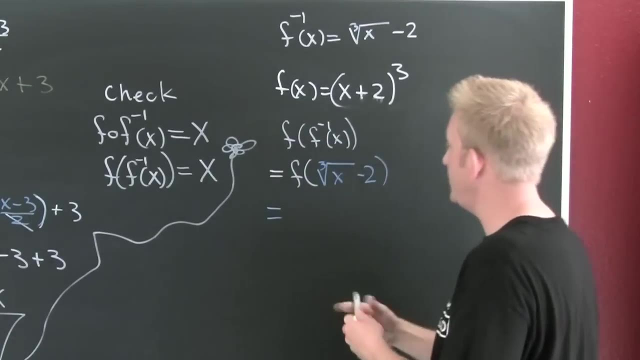 That my inverse was, Uh huh, X minus two. Oh, What does that say? F of f of an x? I see an x. I'm going to put the third root of x minus two. And here we go. This is going to be, This is going to be, Um, The third root of x minus two Plus two to the third. Finish him, Oh.